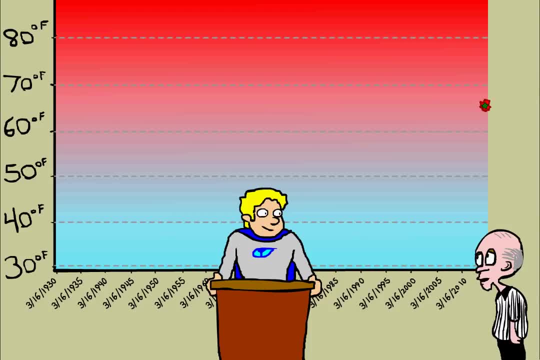 What do you think now? Maybe the high will be in the 60s. Let's add another year. Or maybe the 70s, Except that was an unusually warm year. Let's look at the past 30 years. Okay, With 30 years of data, climate tells us that the high temperature on March 16, 2035 will almost certainly be between 40 and 80 degrees. 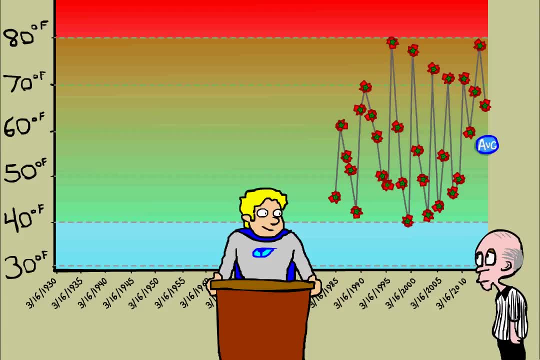 What's the average About? 57?? Yes, And that's the best guess for the temperatures on March 16 next year, Or the year after, Or the year 2035.. At least until you get close enough to predict the actual weather for that date. 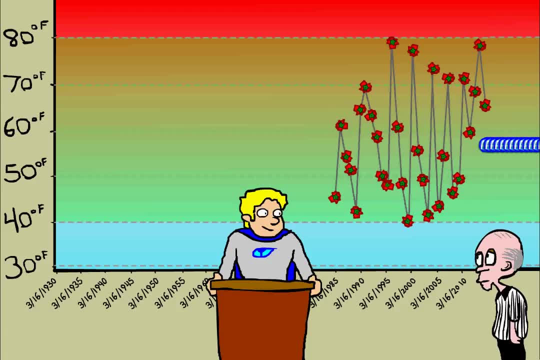 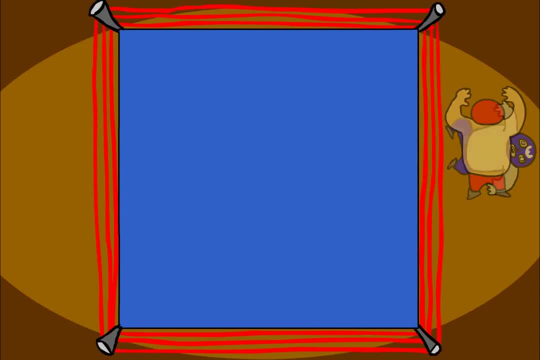 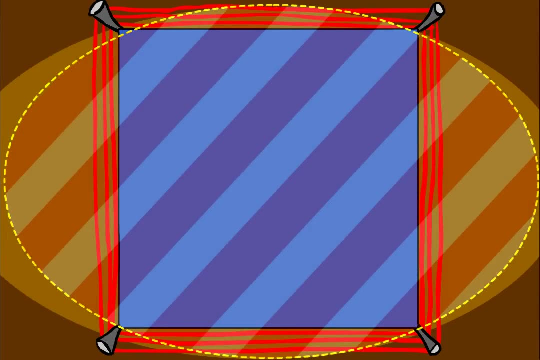 But isn't the climate changing? Yes, Let's go back to our wrestling ring. We might experience an extreme wrestling event that takes us beyond the boundaries of the ring. If this kept happening again and again, we might decide to extend the safety area of our ring, because we expect this kind of thing to happen again. 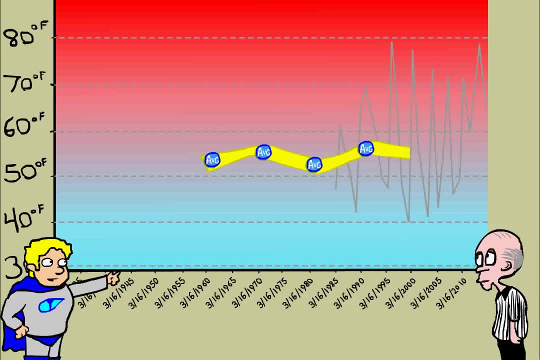 Going back to our data, we can see that the average has changed over time. That's why climatologists usually use a recent 30-year period to get data as close to the current climate as possible. If we look at the high temperatures in St Louis on March 16,- all the way back to 1930, we can see where the average has changed over time. In 1960, looking back at the previous 30 years- the average high temperature was around 54 degrees. By 1970, that average was 55.. In 1980, it was down to 51 degrees. Now that average is up to 55.. 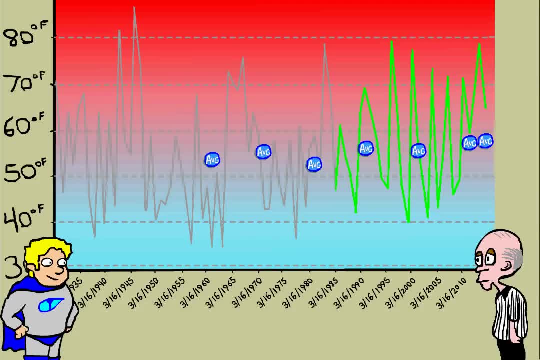 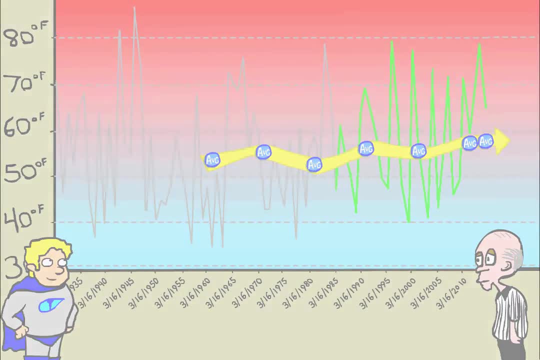 Okay. So if you want to know the climate many years into the future, you need to estimate the changes in the climate too. You can also think about it in terms of time. Climate includes weather over a long period of time. Weather is what's happening now. 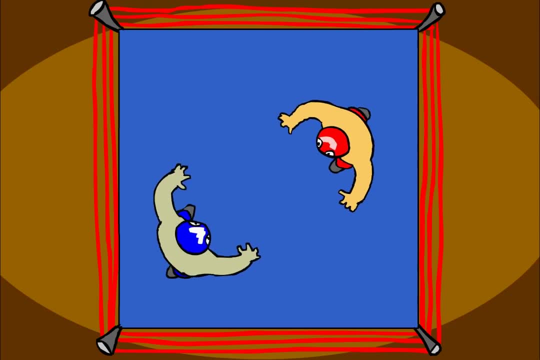 If you were to close your eyes and tell our wrestlers to move around, can you predict where each one is? No, But can you predict that they are somewhere inside the ring? Yes, So, like weather tells me that I can wear a t-shirt today, 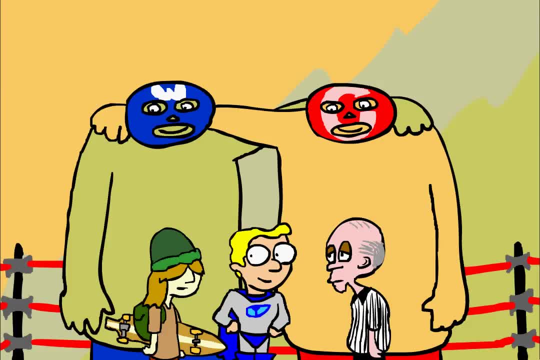 But climate tells me that I better own a rain jacket for all the rain we get. Yeah, you got it. Climate is the upward trend of this stock I bought and weather is the up or down price movement that's happening now. Yeah, that's right. 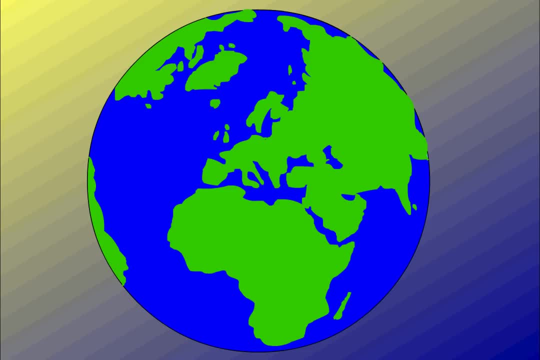 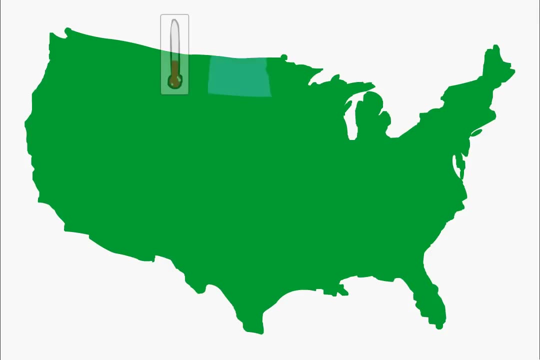 I think you're getting it now. The climate also determines what you can or cannot do. You can't go skiing when there's no snow right. So I may not be able to know the temperature in North Dakota next week, but I could say with some certainty that it'll be colder than Florida. 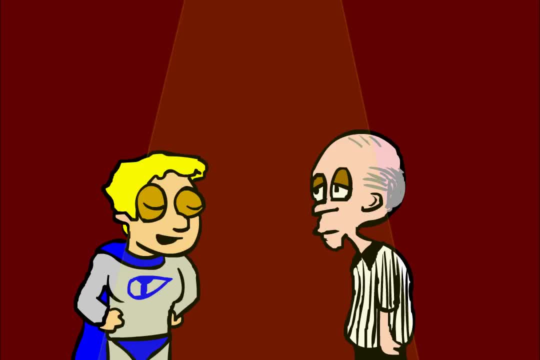 I also wouldn't want to try growing oranges in North Dakota either. Exactly Now you've told us the differences between weather and climate, and we know climate affects what we do. But what determines the climate in the first place? I'm glad you asked. 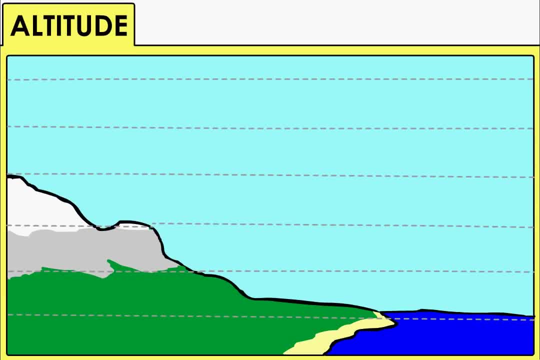 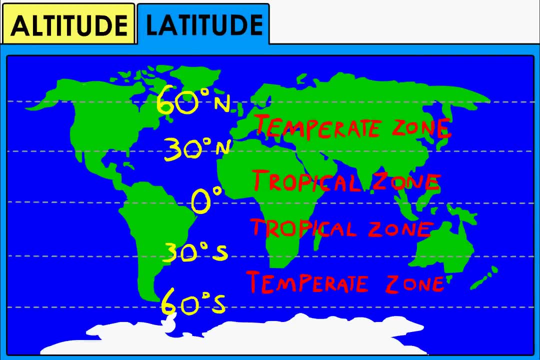 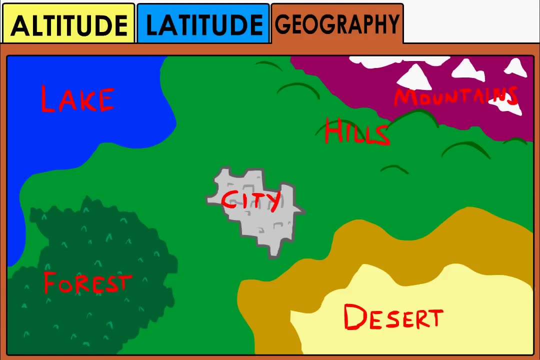 There are four major things that determine your climate. Altitude: Usually, the higher your altitude, the colder it will be. Latitude: The closer you are to the equator, the warmer it gets. Geography: Places near a large body of water results in higher humidity and more moderate temperatures, whereas desert areas tend to be just the opposite. 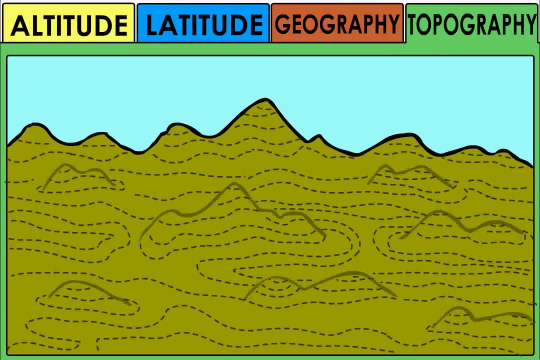 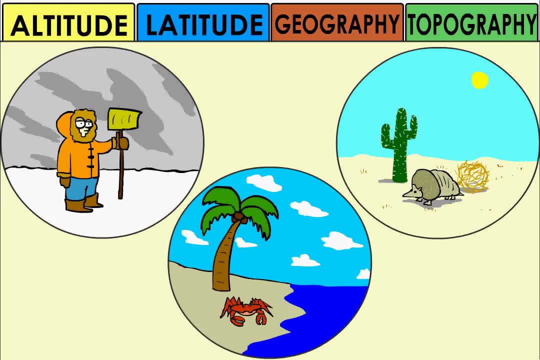 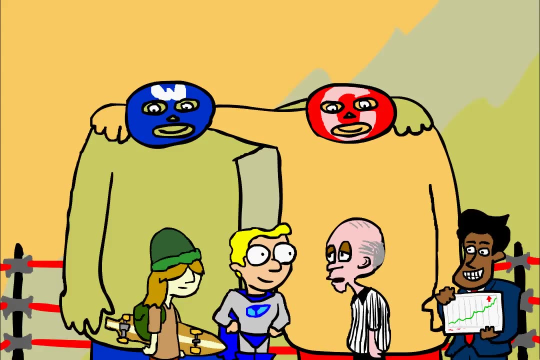 Topography, Mountains can often block the wind, preventing air on the other side of the mountain from affecting the weather. But remember: any given day, any location may experience weather conditions that are unusual for the area, like an extreme weather event. So the climate is what I expect, but weather isn't. 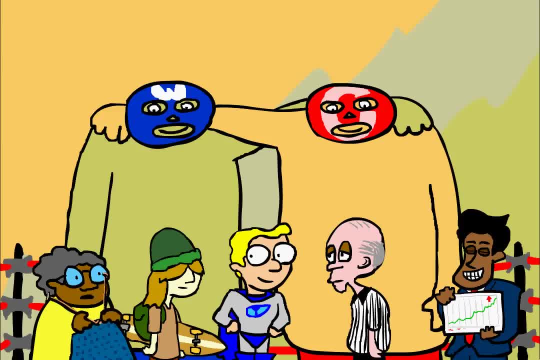 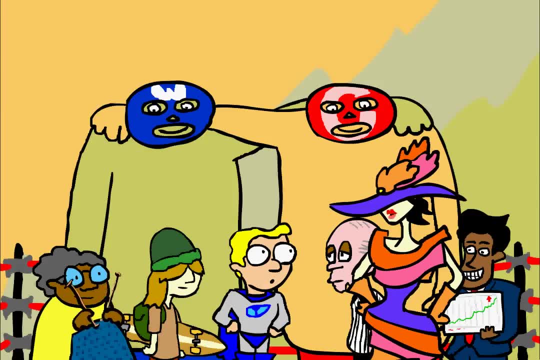 Weather is what I get. Weather is the hook knit I just did, and climate is my afghan. Yes, that's another way too. Weather is the stunning dress on I have right now, while climate is my whole fabulous wardrobe. Okay, I think we get the point. 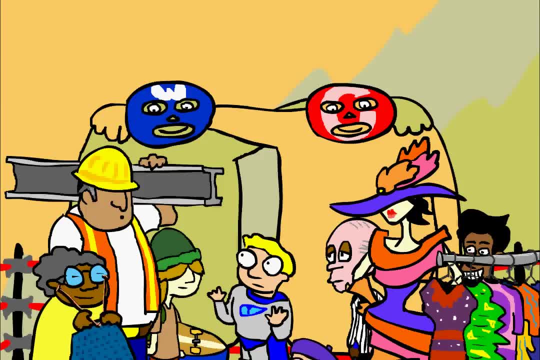 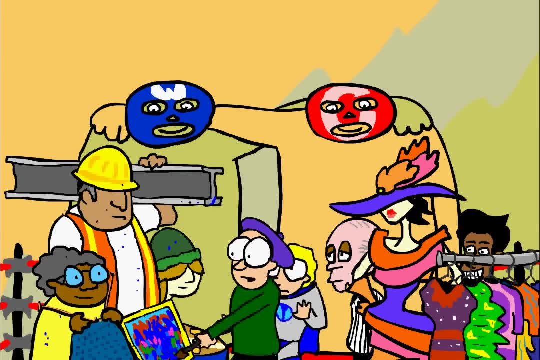 Climate is the whole building I'm working on and weather is the gator I'm about to install. Yeah, I guess, but Climate is my masterpiece painting, But the weather is this stroke and this stroke, and this one, and this one and this one, here, here, here. 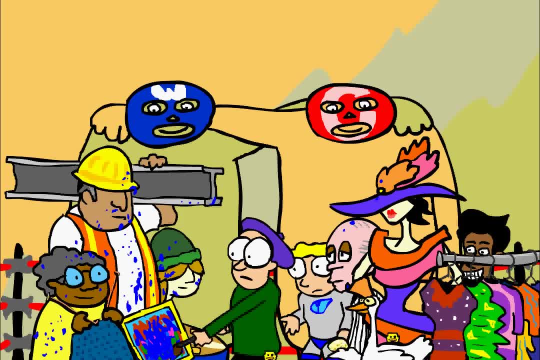 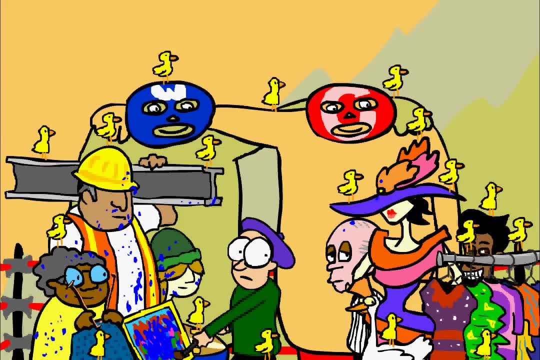 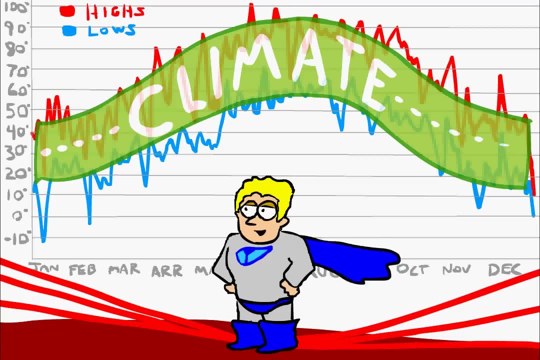 Really, come on. you're getting paint everywhere. It's the egg I'm sitting on now, but climate is my whole family. Now wait just one second. Ducks can't talk, So remember, weather can vary from day to day and climate is the statistics of the environment over time. 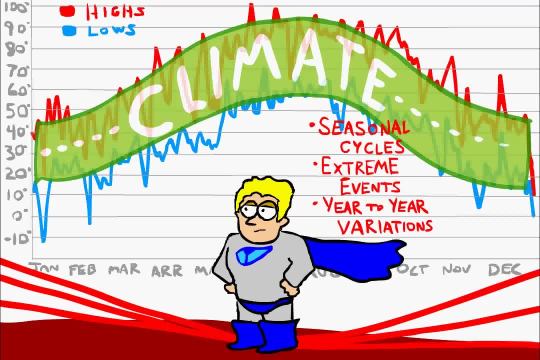 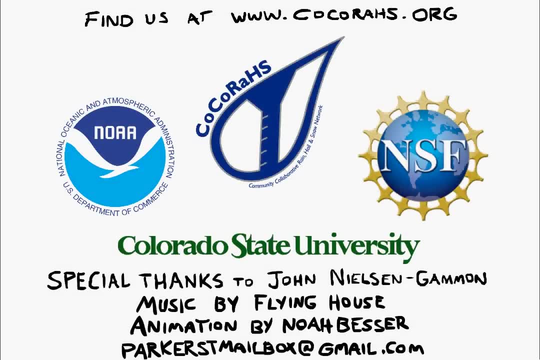 which includes seasonal cycles, extreme events and year to year variations, And that's the difference between weather and climate. Thank you, Thank you.